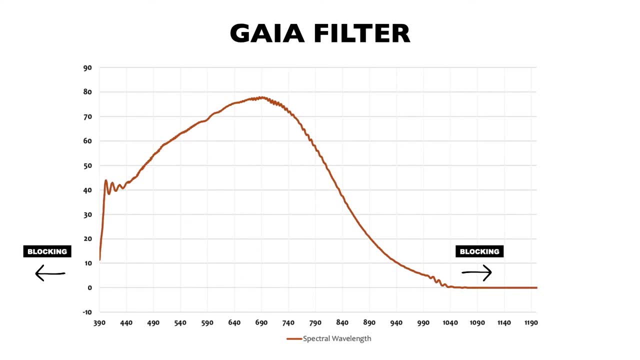 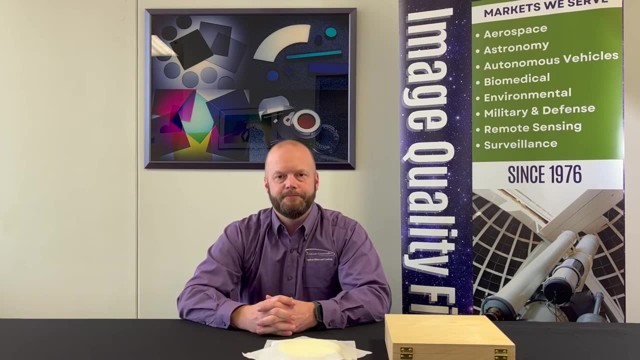 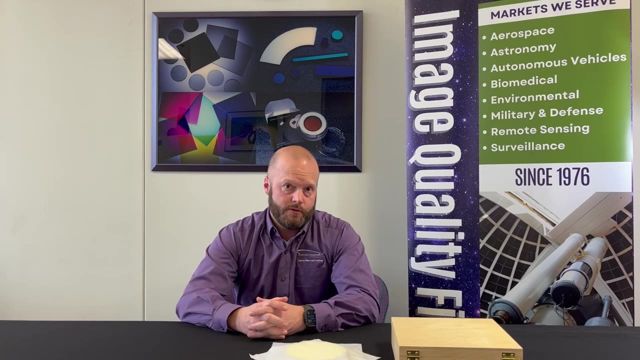 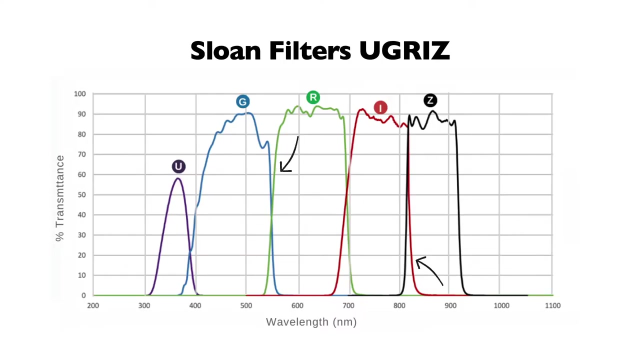 transmits the Cron and John bands, thus eliminating infrared radiation as a pre-filter, before getting to your regular filters. There's also called the Sloan filters. Now, these are very much like the Kron and the John filters, except the crossover between the bands is limited, so you have steeper edges between those bands to create some distinction. 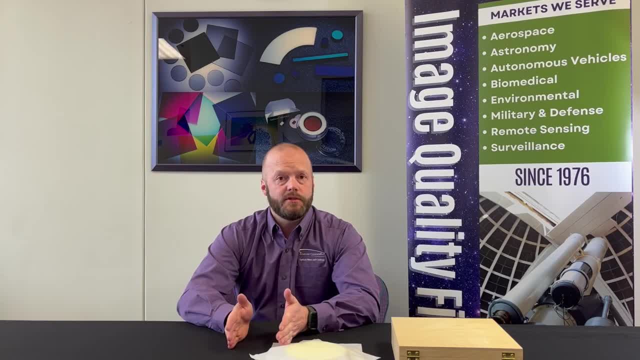 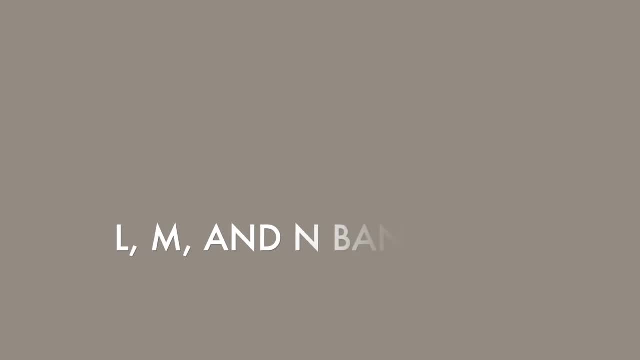 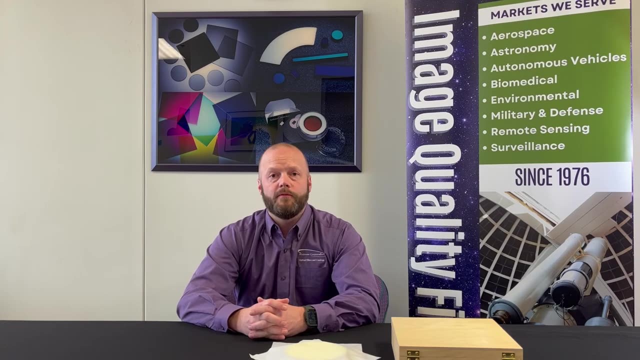 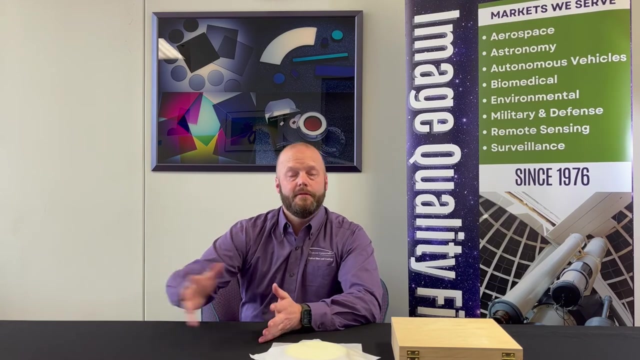 between those color bands. Those type distinctions separate the Sloans from the Kron and John type filters. for whatever your application may be, The astronomical bands don't stop there. They spread into the far infrared as well. The L, M and N band are covered between the far infrared. 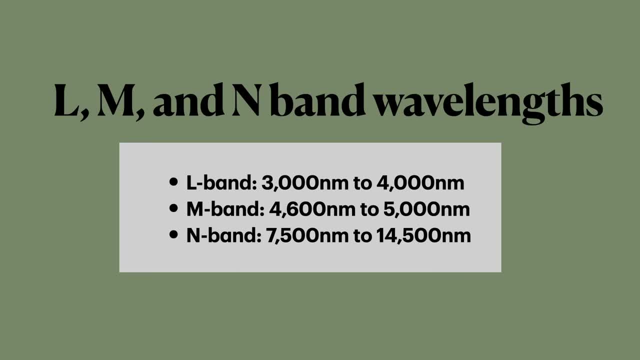 The L and M bands can be combined between, say, 3,000 to 5,000 nanometers, and then the N band is the far 7,500 nanometers to 14,500 nanometers. These wavelength bands have their own purpose. 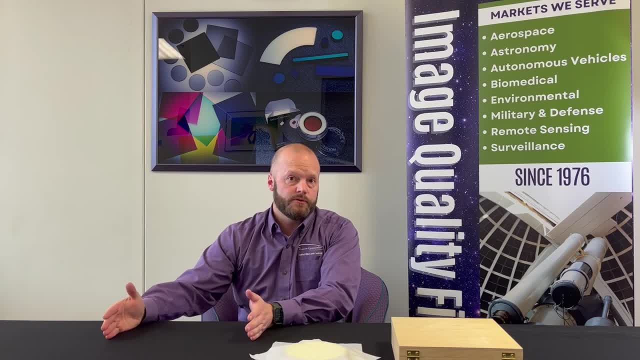 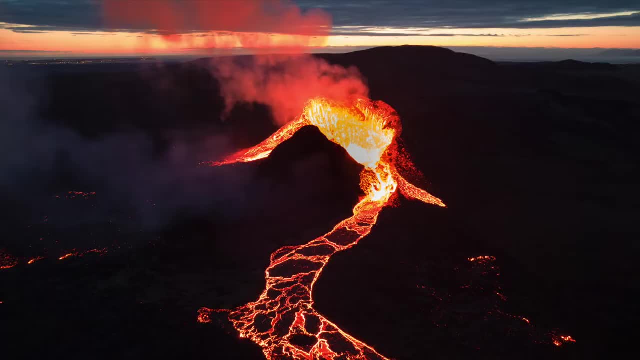 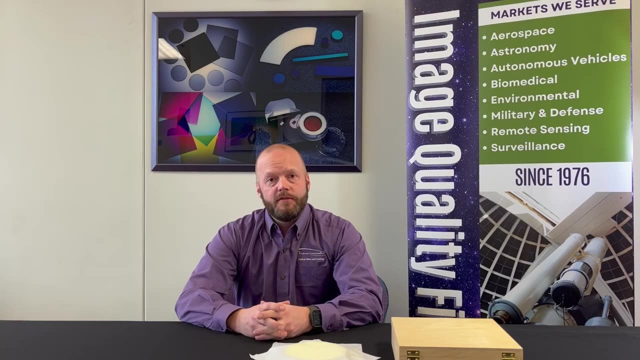 7,500 to 14,500 nanometers, or 7.5 microns to 14.5 microns, are usually hot thermal bodies. Examples are lava flows or, say, an exploding star, things of this nature. Each individual band has its own application that suits whatever the observer needs to. 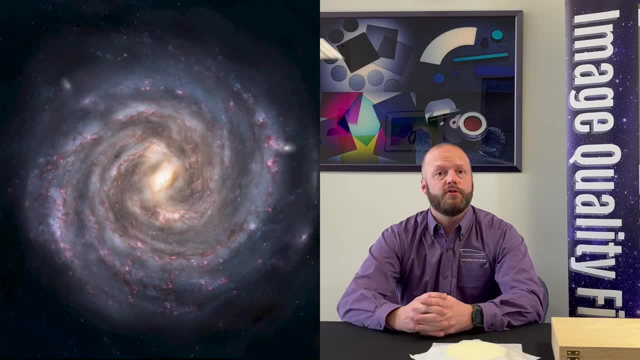 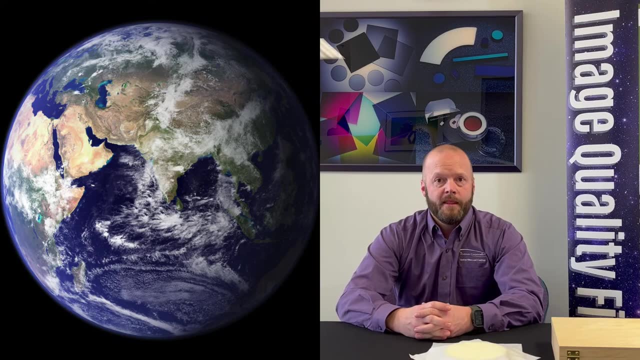 see, We're observing the stars. These bands can also be used to observe Earth by all. We are in the solar system, So the Earth is part of it. Looking down at thermal bodies from, say, small sat and cube satellites in the N band. 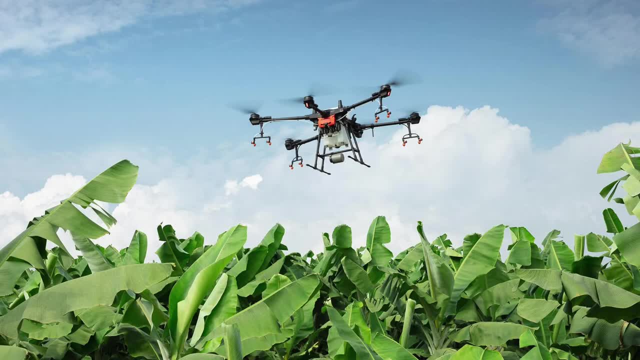 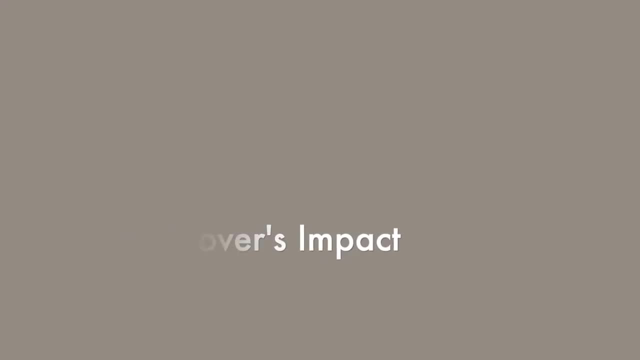 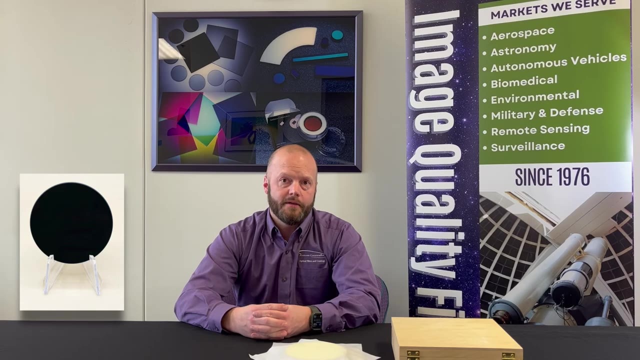